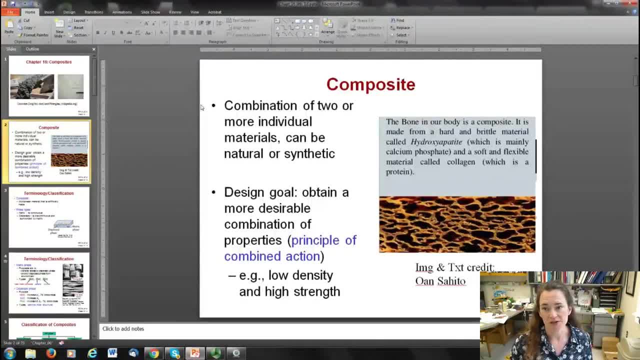 composite is shown here. The bone in our body is actually a composite material. So is wood, by the way. Anyway, bone is made from a hard and brittle material called hydroxyapatite, which is mainly calcium phosphate, and a soft and flexible material called collagen, which is a 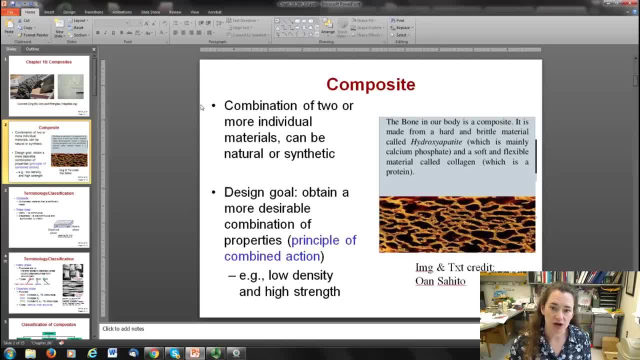 protein. Now the design goal for composites is to obtain a more desirable combination of properties. This is actually called the principle of combined action, when you combine properties of two different materials to become a better, more desirable combination for whatever you're trying to do. For example, you might want a low density material that's also high strength, Like, say, 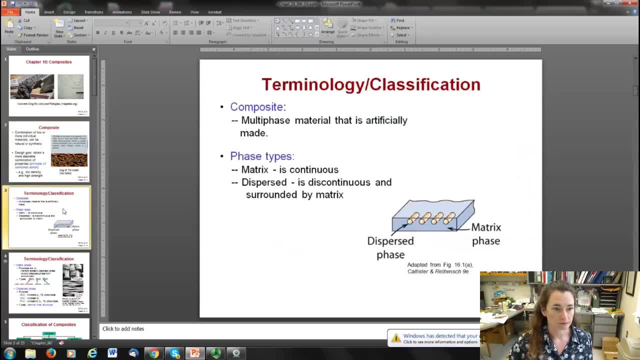 for example, a carbon fiber. You might want a low density material that's also high strength. Now, composites are multi-phase materials and a lot of them now are artificially made for various structures and building materials. You have two phase types, at least in a composite material. You 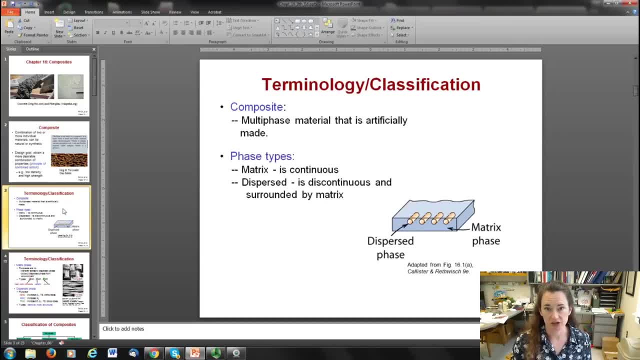 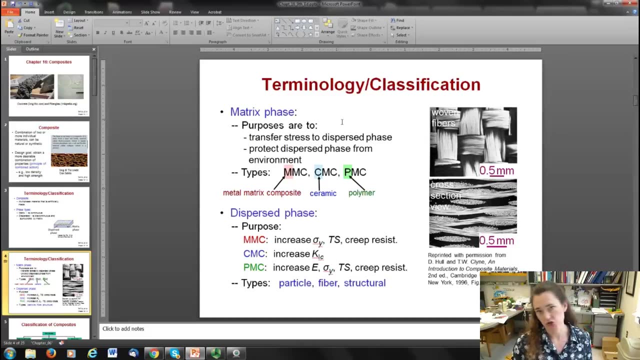 have your matrix and that's your continuous material. that kind of binds it all together. And then you have your dispersed material. It's discontinuous and it's surrounded by the matrix. The purposes of your matrix phase are to transfer stress to the dispersed phase, which is usually your strong material. 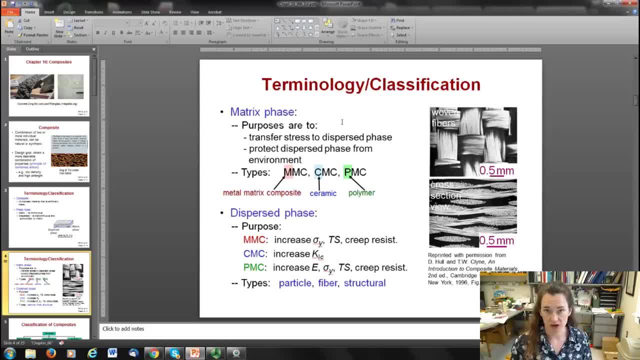 and it also protects the dispersed phase from the environment. So some typical examples are metal matrix composites or MMCs, ceramic matrix composites or CMCs, and polymer matrix composites or PMCs. The dispersed phase can serve a variety of purposes. It can increase your yield strength. 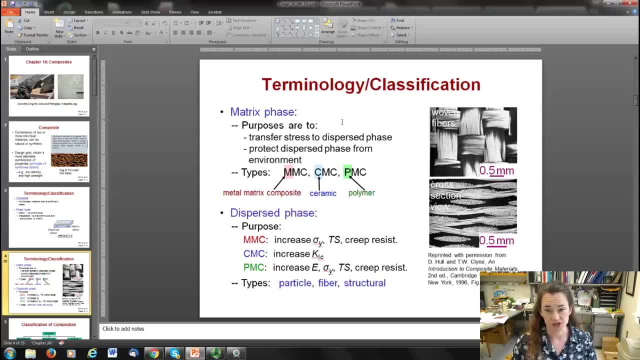 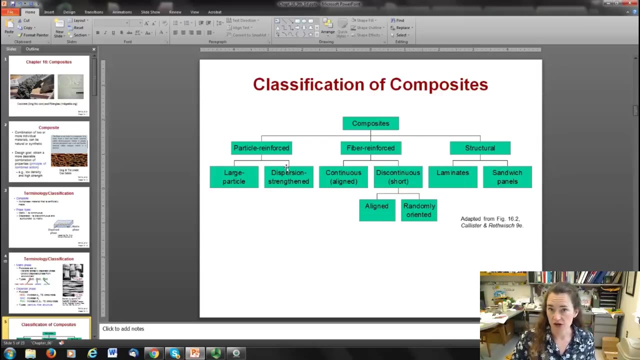 increase your tensile strength or increase resistance to creep. It can also increase your fracture toughness or increase your elastic modulus. It comes in three types. It can be particles, fibers or structural for the dispersed phase. Here's some of the classification of these composites, So of the three that I already said, 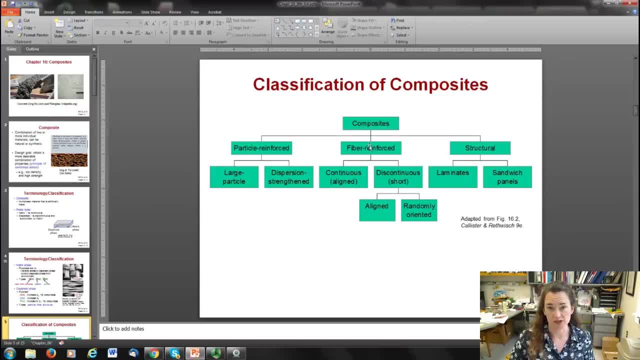 the particle reinforced, the fiber reinforced or the structural composite. they can have subdivisions. So under particle reinforced you can have your large, large particles, like a cement, for example, or a concrete in cement, Or it can be dispersion strengthened with small particles that are in the order of 10 to 100 nanometers, Your fiber. 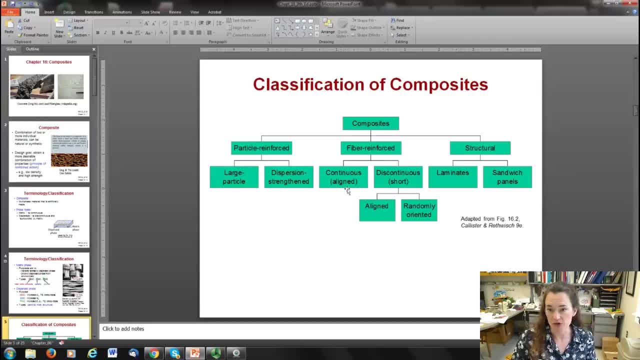 reinforced can be continuous, which means long fibers and they can be aligned, Or they can be discontinuous fibers, meaning that they can be very short, And among the discontinuous, they can be either aligned or randomly oriented. And your structural composites 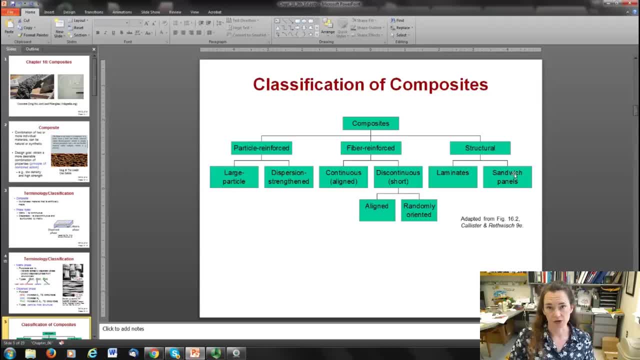 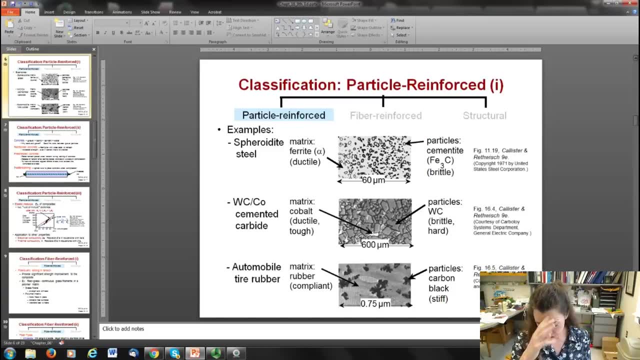 for example, can fall under two broad categories: the laminates and the sandwich panels, which we'll talk more about later. So here's some examples of your particle reinforced. So at top here we have one that we kind of already covered, the spheroidite steel, So that one has the matrix of 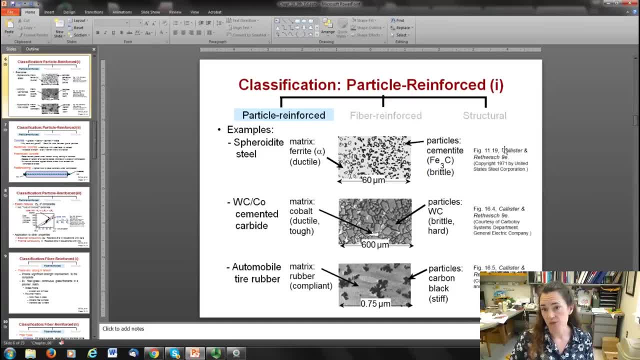 the ferrite, which is the alpha phase, and it's more ductile. And then the particles are cementite, and those are brittle and hard. So in this case, your matrix being embedded with these little cementite particles, the cementite particles themselves actually act as barriers to slip. 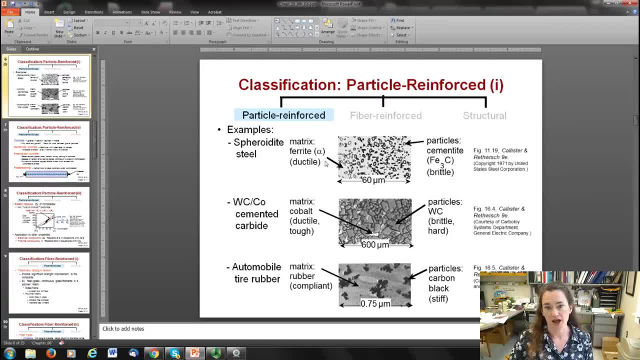 which makes the material harder than the alpha phase would be by itself. The next example here is the cemented carbide. This is actually often called a ceramic metal composite or a cermet. The one shown here is a large particle, and here you have your tungsten. 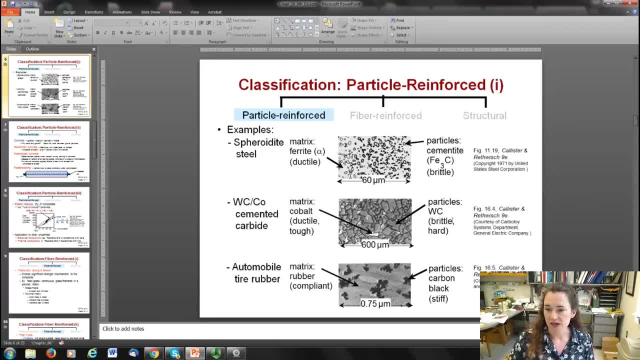 carbide particles in your cobalt matrix. In this case, you have a large particle and you have a tungsten carbide. So in this case, your tungsten carbide particles are very brittle and hard, whereas your matrix, the cobalt, is more ductile and tough. Now, in particular, this composite is 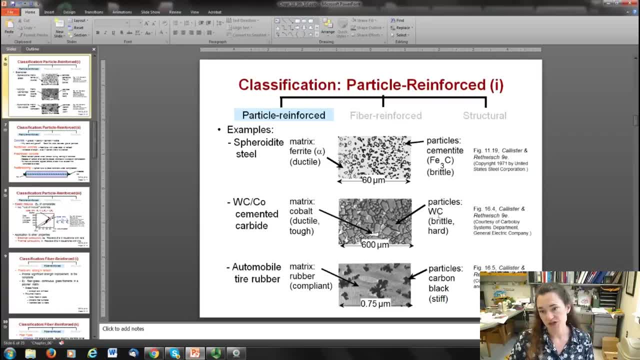 often used for cutting steels. The tungsten carbide particles are really brittle and hard. If you tried to cut the steel with just the tungsten carbide without being in the matrix, it would probably fracture because it is so brittle And so the cobalt provides. 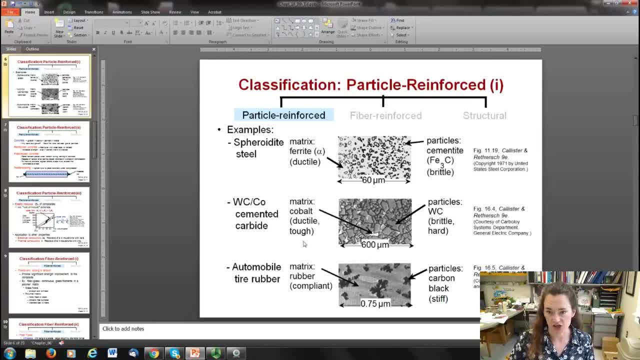 um ductility and toughness to the material that prevents fracture. And then here at the bottom, there's automobile tire rubber, which is a matrix of rubber which is compliant, and uh sort of springy material combined with carbon, black Carbon. 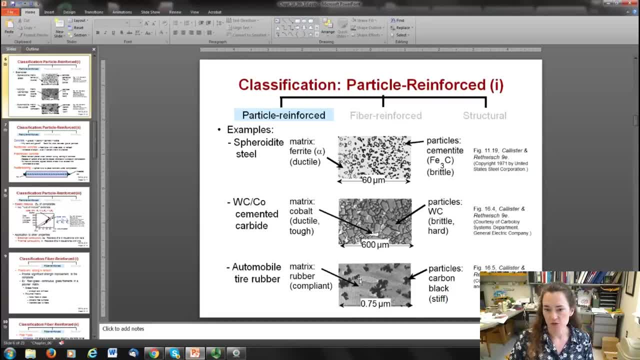 black is what you get when you burn hydrocarbons and it forms these little, almost spherical particles that are small. This is an example here. the automobile tire rubber is an example of the dispersion strength And um composite, because you can see here these little carbon black particles are very 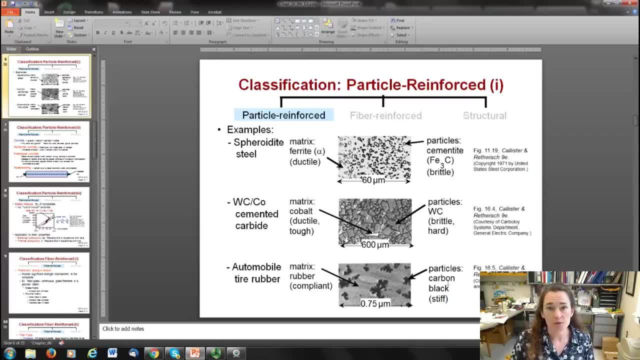 small. What happens is when you add the carbon black to the rubber, the tire becomes a lot more tough and resistant to tears and, uh, a lot harder material than it would be without the carbon black. Oftentimes tires are about 15 to 30% by weight um carbon black material. 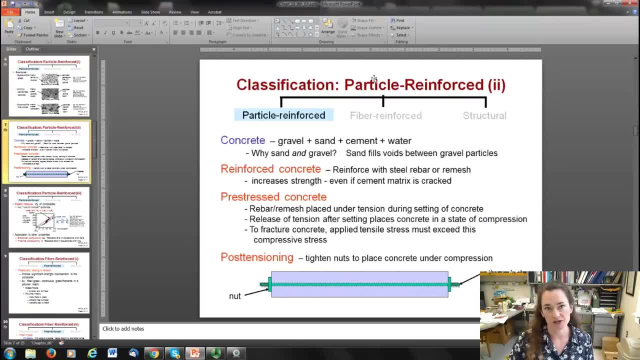 Another really common material that we talk about is concrete, In terms of uh, composite materials. I've actually posted several videos about concrete, because it is one of the more important and commonly used composite materials on the planet. So concrete is not the same as cement. Um, concrete is actually a mixture of gravel and 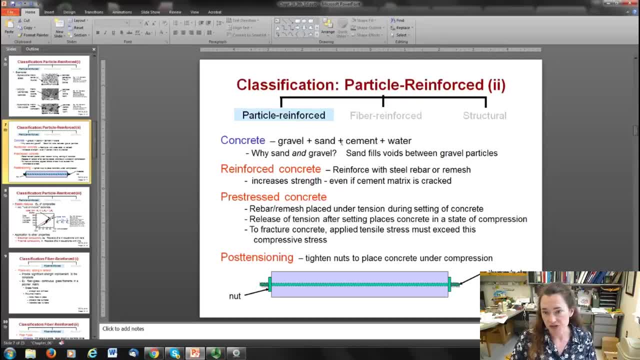 sand and cement. So concrete is gravel, sand, cement and water And the sand and gravel actually fill the voids between the gravel particles. You can reinforce concrete with steel rebar or remesh and that increases the strength so that even if the cement matrix 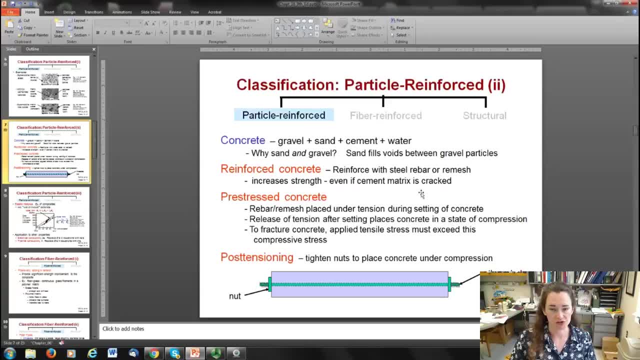 cracks over time, the material still stays strong and supports the load. You can also pre-stress your concrete by putting a rebar or a remesh and placing it under tension while the concrete sets, And then the release of tension after setting places the concrete. 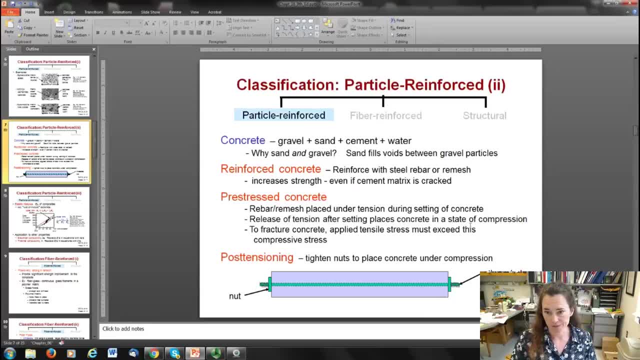 in a constant state of compression which makes it stronger, And to fracture concrete and apply tensile stress has to exceed the compressive stress. So concrete is a very important material that we talk about. So concrete is a very important material that we talk. 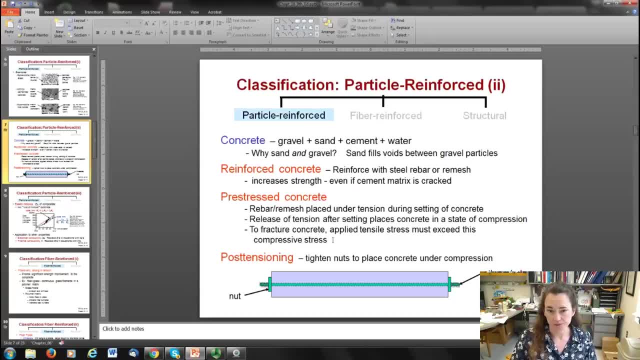 about, And so concrete is a very important material that we talk about, And so concrete is a very important material that we talk about, And so concrete is a very important raw material that we look at to determine the compressive stress that it's already in. You can also. 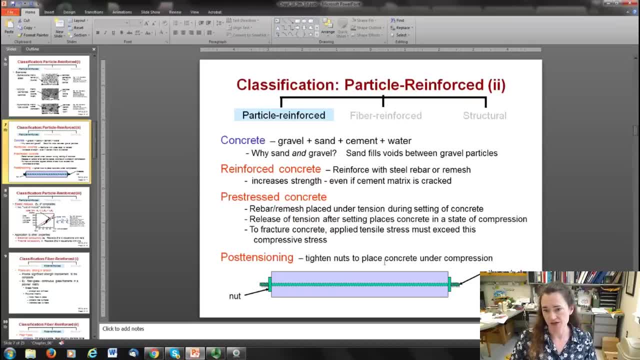 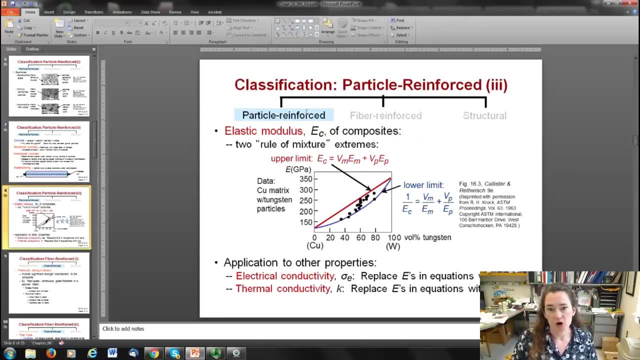 post-tension it by putting nuts on the ends to place the concrete under compression. Now, moving on to the particle reinforced formulae for the elastic modulus. You can see here that the elastic modulus E for the composite with the subscript sub-C can. 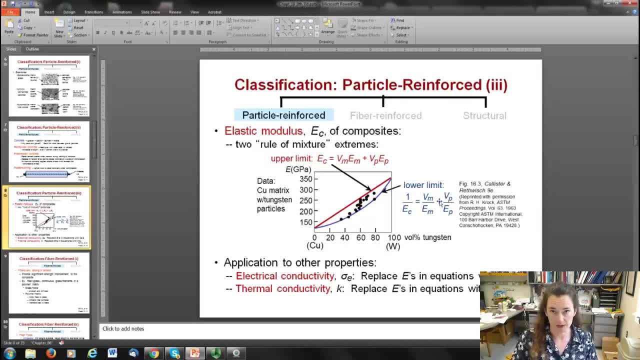 be put between an upper and a lower limit, OK, and this is actually known as the rule of mixtures. between then, it says that your material property for your matrix, your sub m here, your m subscript here, and your particulate p, the p subscript here. 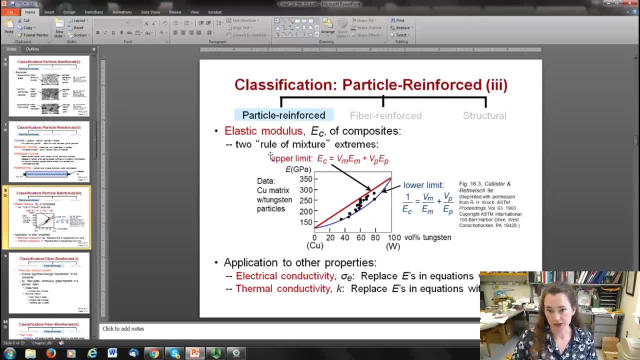 is actually going to be a mixture and it will fall between the upper limit equation- here e sub c is equal to vm times em plus vp times ep. here v stands for the volume fraction and e stands for the modulus, as I said- and then the lower limit expression is 1 over ec. 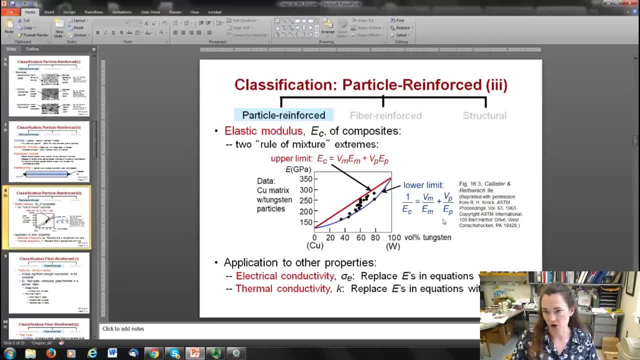 is equal to vm over em plus vp over ep, and so you can see here: the expressions for the upper and lower limits are shown here in red and blue and the values, the actual values, for this composite material fall in between the upper and the lower limits according to the rule of mixtures. 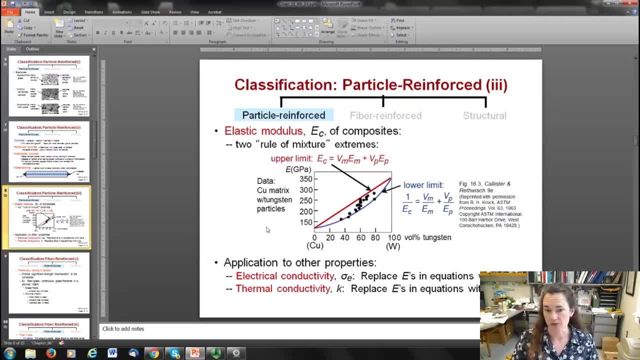 this expression can also be applied to other properties, not just the modulus, for example, but it could be used to express the electrical conductivity, where you replace the e's in the equation with the sigmas for the conductivity, or the thermal conductivity k, where you replace the e's with k's. 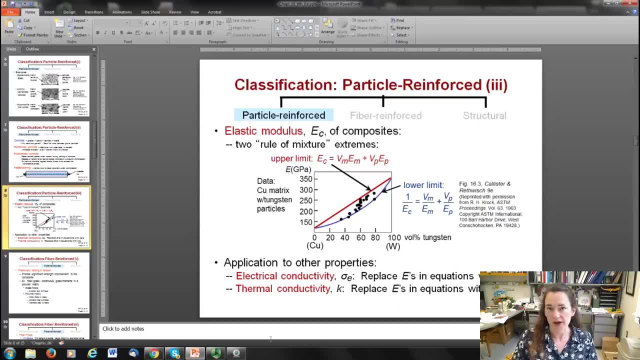 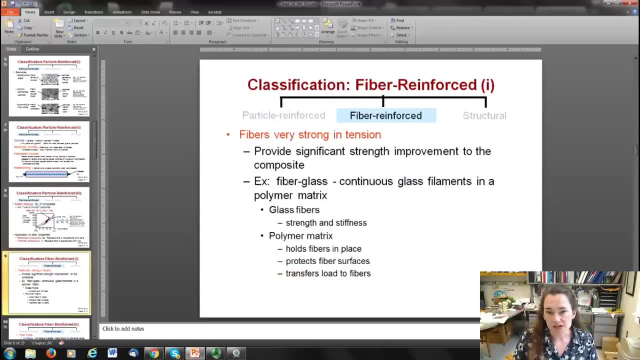 so it gives you a good expression, general expression, for estimating what the material properties of a composite would be. now the next classification of composites is actually technologically probably one of the most important types of composites, and that's fiber reinforced composites. and fibers are very, very strong in tension, so they provide significant 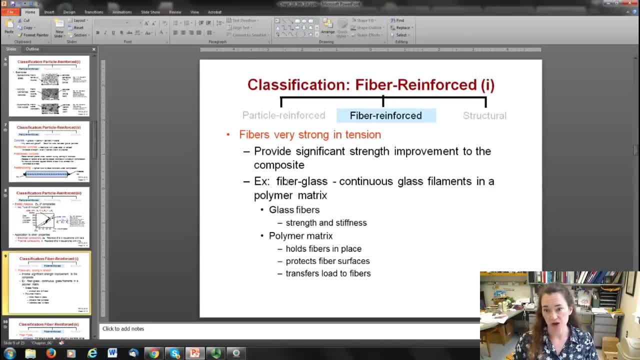 strength improvement to the composite. for example, you might be familiar fiber glass, which is continuous glass filaments in a polymer matrix. there the glass fibers provide strength and stiffness, while the polymer matrix holds the fibers in place, protects the fiber of surfaces and transfers load to the fibres. 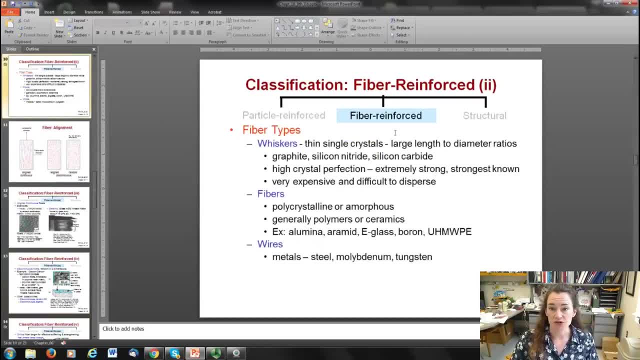 you can have different fibers of fiber like this. you can have different fibers of fiber like this. fibrous fiber consists of fiber 6 and x and x. fibrous fiber consists of fiber 6 and x and x different fiber types. one is whiskers, which are thin single crystals with 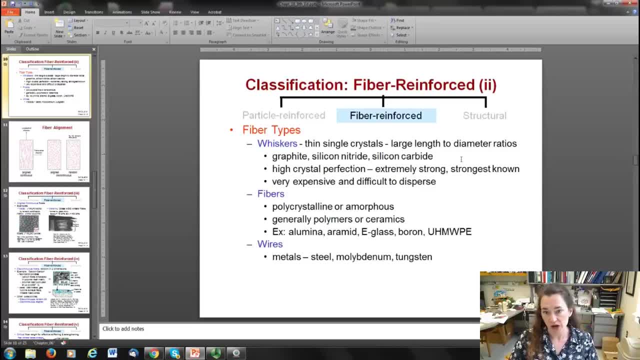 large link to diameter ratios, and some examples of those are graphite, silicon nitride, silicon carbide. there's also some of those that are being applied to nanotechnology, where you have carbon fiber and carbon nanotube whisker type fibers. they have a high crystalline perfection, these whiskers, they're. 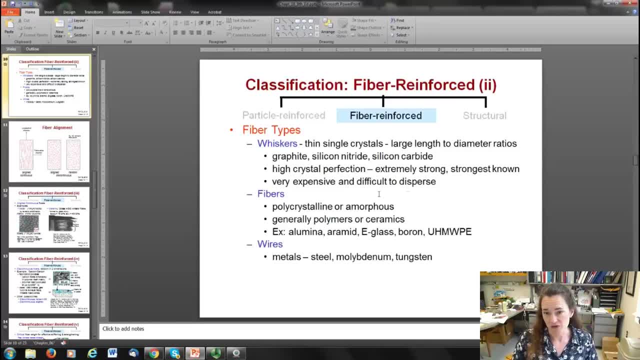 extremely strong. in fact, they're the strongest known. however, they can be very expensive and they can be difficult to disperse. you can also have fiber, fiber types which are polycrystalline or amorphous, and those are generally polymers or ceramics, for example, alumina, aramid, glass, boron, ultra-high molecular 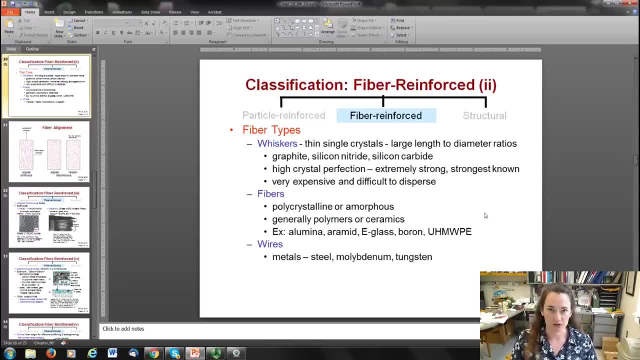 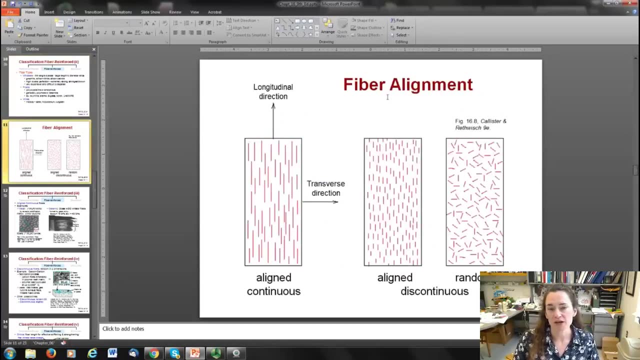 weight polyethylene. those are all fibers that can be used in these composites. and then, finally, you can have wire fiber types. those are metals like steel, molybdenum and tungsten, and those provide strong resistance to creep you. The way the fibers are aligned really dictates a lot of their performance. 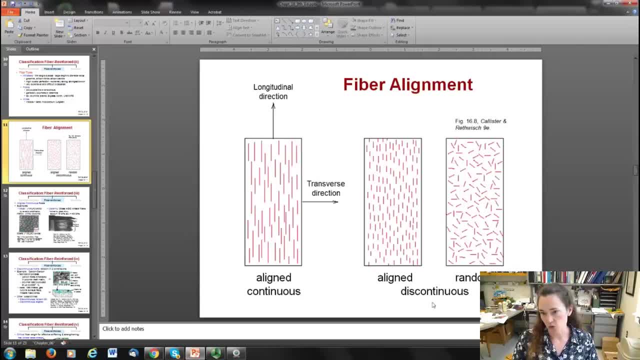 There's two types. There's the aligned continuous or the discontinuous. Remember, the continuous are the long fibers, very long fibers- They're about 30 times the critical length, which is a property that we'll get to in a minute. And these continuous fibers, because they are long, they basically have to be. 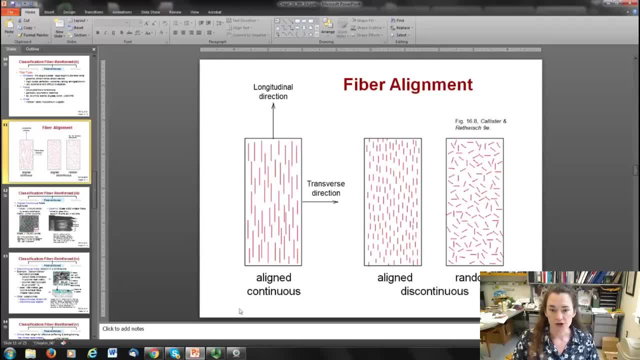 aligned in the longitudinal direction. So here you have longitudinally aligned fibers. The performance of these aligned continuous fibers can be very different depending upon which direction the stress is applied. If it's applied in a longitudinal direction, they'll be much, much stronger. 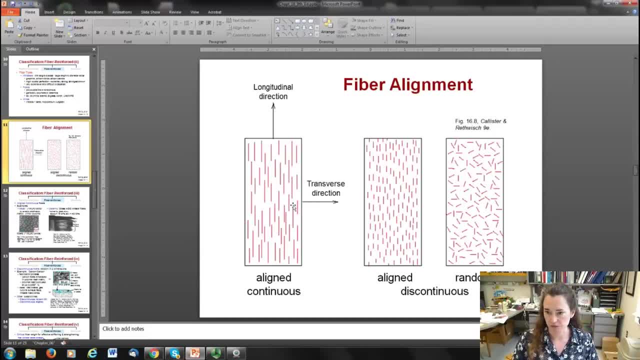 than if the stress is applied in a transverse direction. For the discontinuous or short fibers you can either have aligned or random orientation of the fibers. You might want random orientation if you're not really sure what direction the stress is going to be applied in or if it's just as likely. 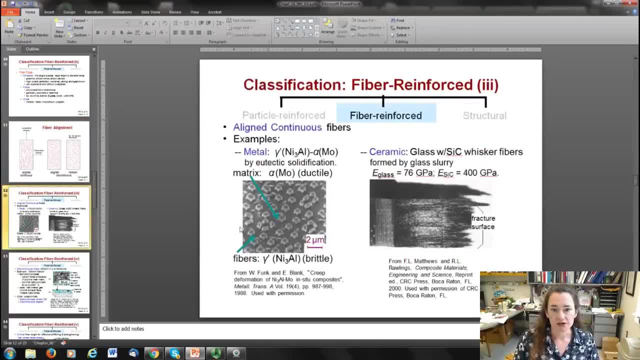 the stress could come from any direction. Here's some examples of the fiber reinforced composites, some images of what they might look like. For example, here's the metal wires type composite and you can see here that you have these metal fibers embedded in a metal matrix and that provides a strong resistance to creep. 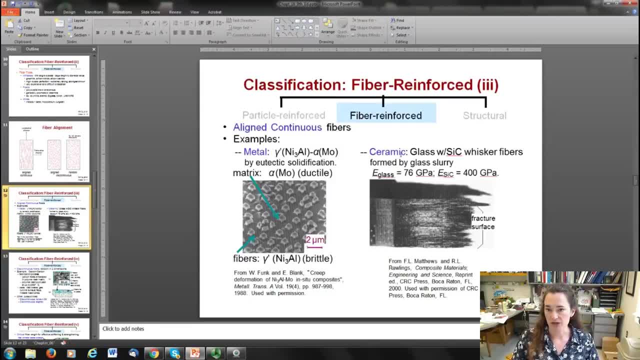 and also more strength. You can also have here an example of ceramic with glass, with silicon carbide whisker fibers, and that's formed by a glass slurry, And you can see that there's actually a pretty big spread in between the elastic modulus for the glass or for the silicon carbide. 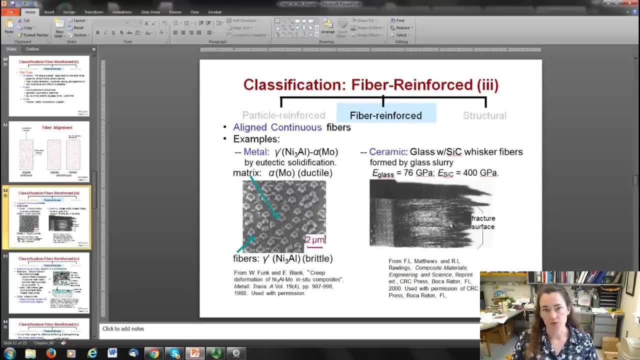 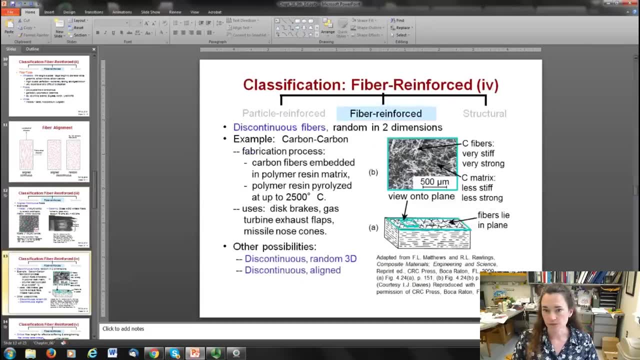 And so you would get a much stronger and much higher elastic modulus for the material when you mix those fibers in. Here's some examples of some discontinuous fibers. This one shows an example of carbon fibers embedded in a polymer resin matrix. These can be used in disc brakes, gas turbine, engine flaps and nissl nose cones. 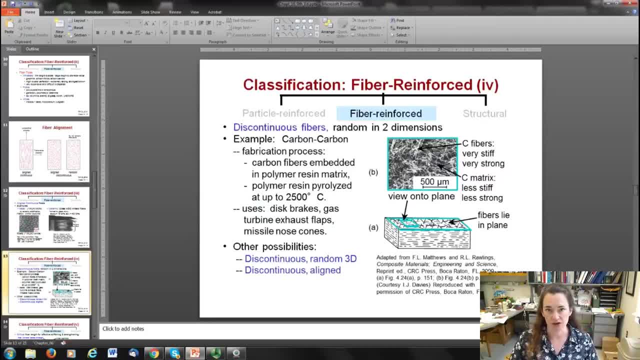 I've actually posted another external video on carbon fibers because they are one of the more important new types of composites out there and I encourage you to watch that Also. you can have the fibers aligned in the plane or they could be aligned randomly in. 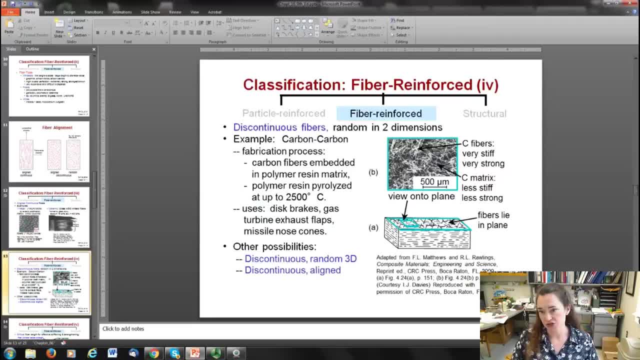 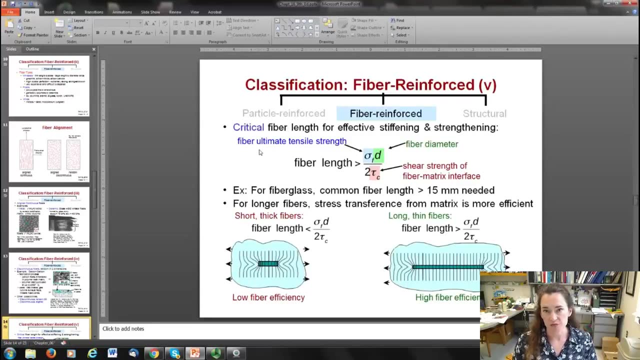 three dimensions or they could be aligned. So in the images that's shown here this is random in two dimensions, but aligned along the plane. Now, the length of the fiber that you use is very, very important for the fiber's performance. 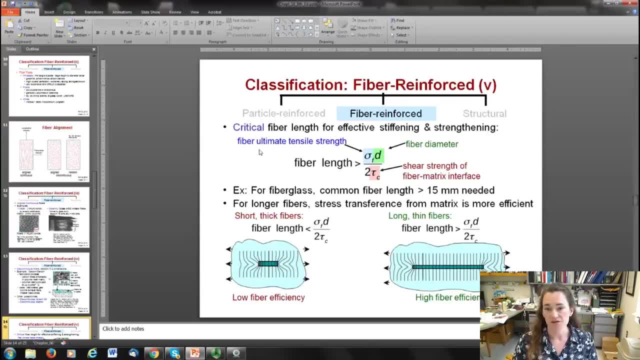 So there's something called the critical fiber length for effective stiffening and strengthening. You're actually not going to get significant strengthening or stiffening unless the length exceeds the critical length, sometimes by quite a lot, But the expression for the critical length is given here. 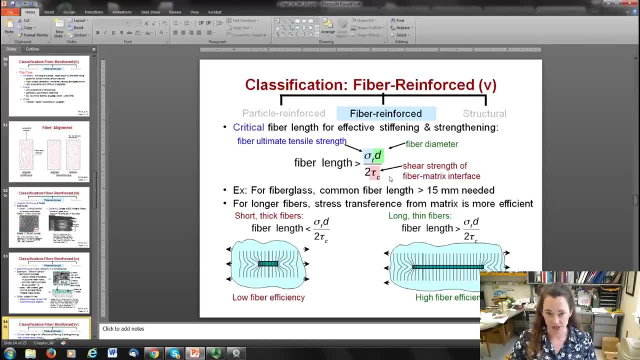 It's sigma f times d over 2 times tau sub c. Here sigma f is the fiber's ultimate tensile strength, d is the fiber diameter and tau sub c is the shear strength of the fiber matrix interface. So, for example, for fiberglass a common fiber length greater than 15 millimeters is needed. 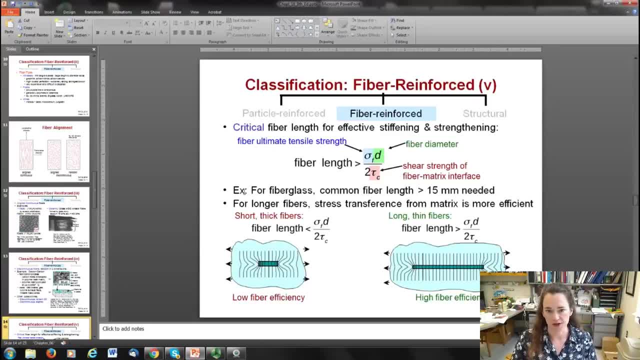 and a typical is 1 millimeter- might be for the critical length. For the longer fibers the stress is transferred from the matrix more efficiently and so you have a stronger material. So for a long thin fiber where the length is much greater, 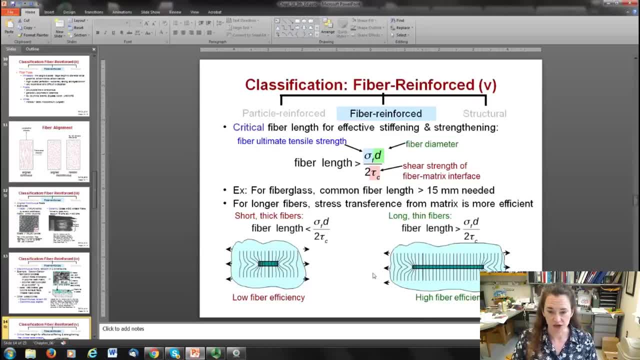 than the critical length, then you have a high fiber efficiency, whereas if it's less than the critical length, then the efficiency of the fiber is much lower and it acts kind of more like a particle composite when it's less than the critical length. 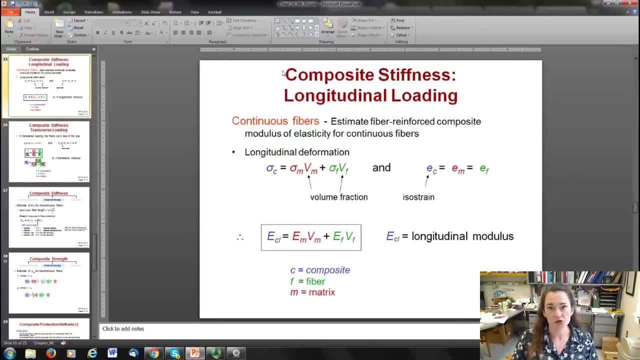 Now, when you place the fiber under longitudinal loading- for a continuous fiber, for example- that means that it's a very long fiber and the axis of the orientation of the fiber is called the longitudinal axis. When you place it under that, you can get significant strengthening of your material. 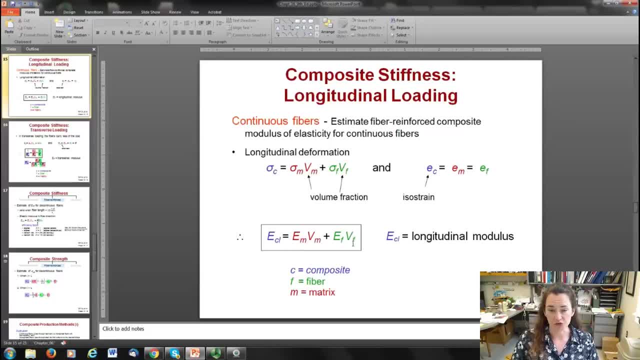 The expression for quantifying what the elastic modulus is is shown here: E is the elastic modulus and V stands for the volume fraction. So E for the composite material when it's under longitudinal is E sub cl and that's the elastic modulus when the composite fiber is under it being loaded longitudinally. 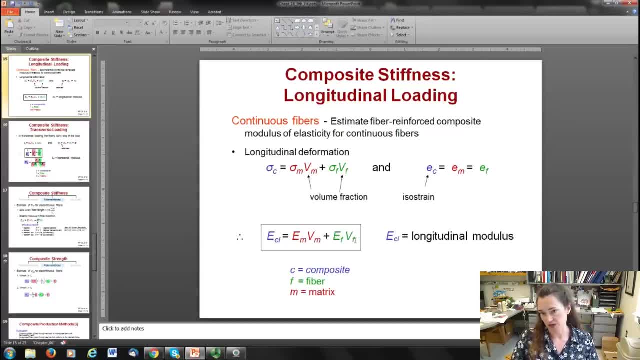 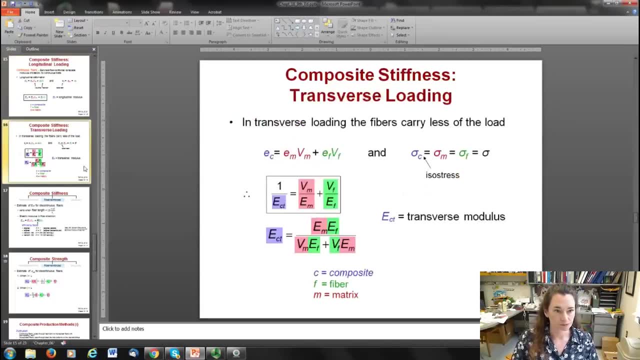 And that's equal to E sub m times V sub m plus E f times v. Here f stands for the fiber and m stands for the matrix. When it's loaded transverse, the fibers carry much less of the load. so the strengthening 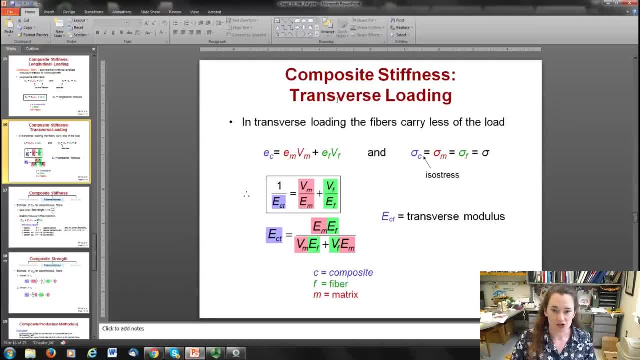 in the transverse direction isn't very much. It's actually a comparable expression to what the lower bound for a particle is, as we went over later And that's shown here For transverse loading. you have 1 over E sub ct. 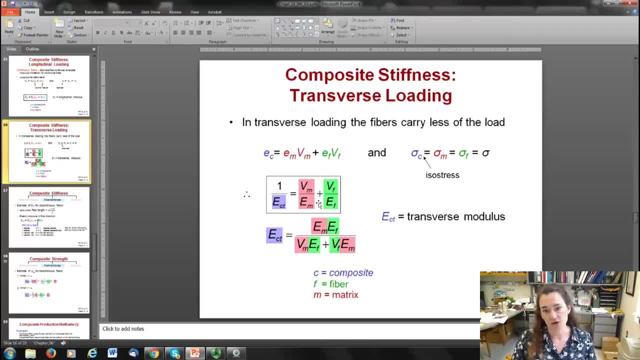 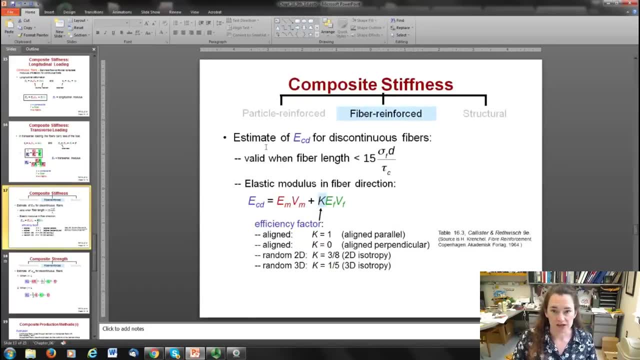 T here stands for transverse, And that's equal to 1 over E sub ct. V here is equal to Vm over Em, plus Vf over Ef. Now you can estimate what the elastic modulus for a composite for discontinuous fibers are. 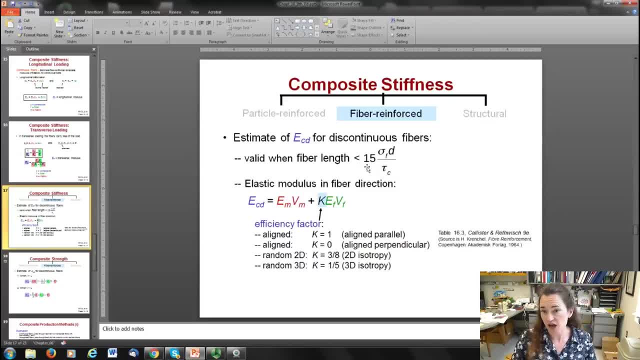 And this is valid when the fiber length is less than, say, 30 times the critical length, or 15 sigma fd over tau sub c. In that case the expression looks like this: E c sub d. right Here E is the elastic modulus again. 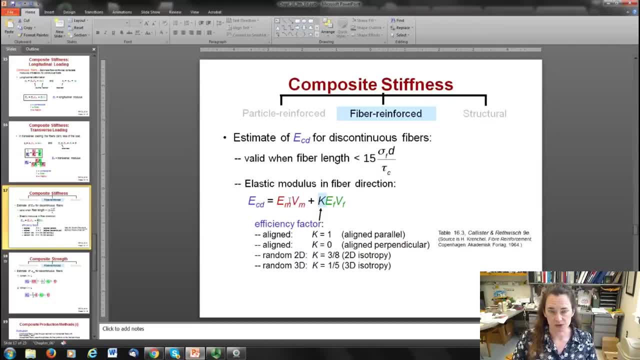 C stands for composite and D stands for discontinuous, is equal to E sub m, V, sub m plus K, E, F, V, F. K is actually an efficiency factor that ranges between 0 and 1.. The value is 1 when the fibers are all aligned and parallel to the longitudinal direction. 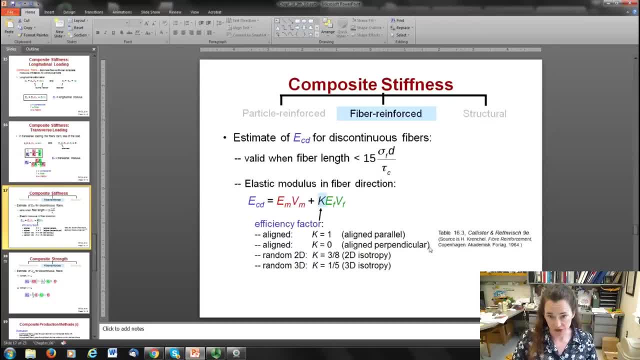 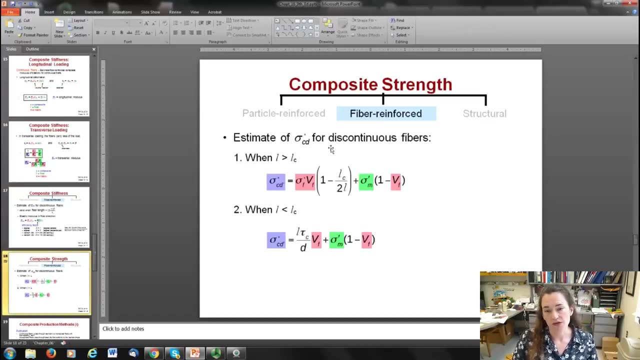 and K is equal to 0 when it's aligned and perpendicular. If it's random in two dimensions, K is often 3 eighths, and if it's random in three dimensions, K is often 1 fifth roughly. This is an expression for the tensile strength for discontinuous fibers. 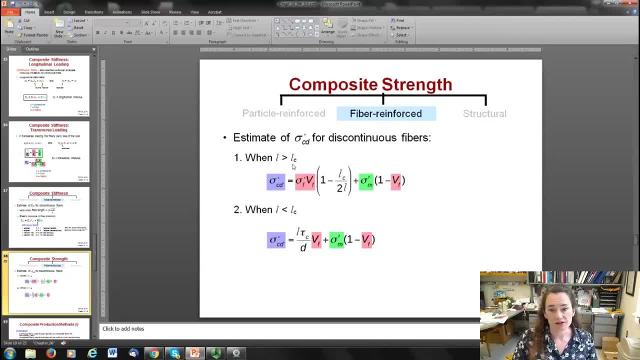 The tensile strength here is given by sigma. When the length is greater than the critical length, then sigma star C sub D is equal to sigma F star times V F, where V F is the volume fraction and sigma F is the volume fraction. 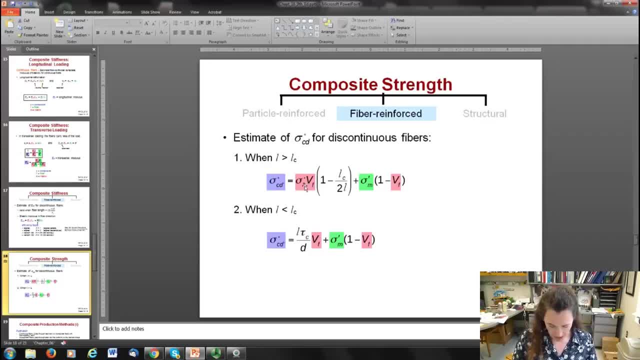 sigma F is the volume fraction and sigma F is the volume fraction. sigma F is the tensile strength of the fiber. and then we have that times 1 minus L C, where L C is the critical length over 2, L, where L is the actual length plus sigma M. 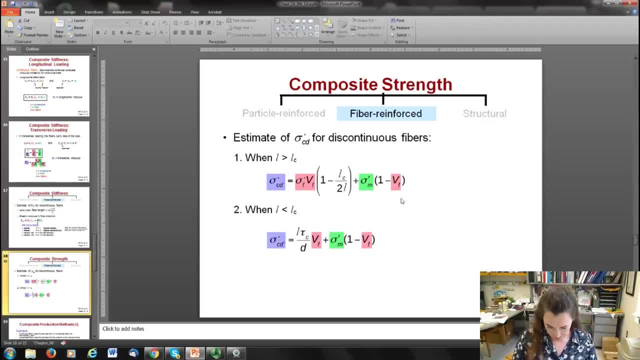 prime times 1 minus V F. Now here, when L is less than the critical length sigma sub C, D star is equal to L times tau sub C over D times V F, plus sigma M, prime times 1 minus V F. Now here the D stands for diameter. of course, L stands for the length tau sub C is going. 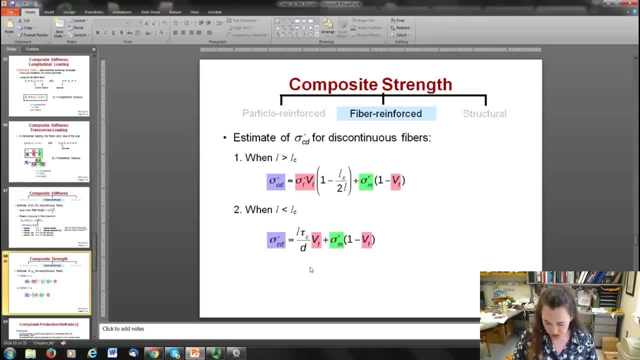 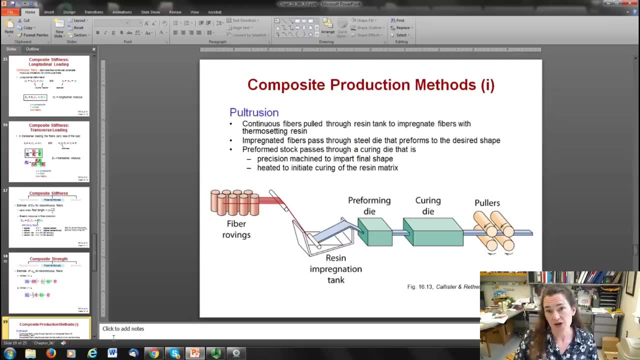 to be the smaller of either the fiber matrix bond strength or the matrix shear yield strength. And, if I didn't say it before, the sigma M prime is the stress in the matrix when the composite fails. There's a few videos, too, actually, that I've posted on composite production materials. 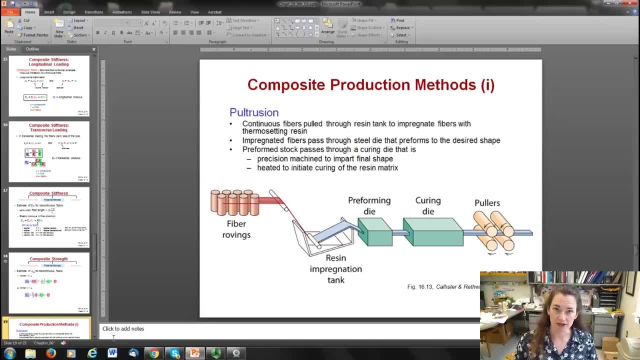 and I really encourage you to watch it because it shows you what's happening. It shows you what's happening inside the factory and it's really pretty interesting. But one of the more common production methods for composites is called pultrusion. That's when continuous fibers are pulled through a resin tank to impregnate the fibers with 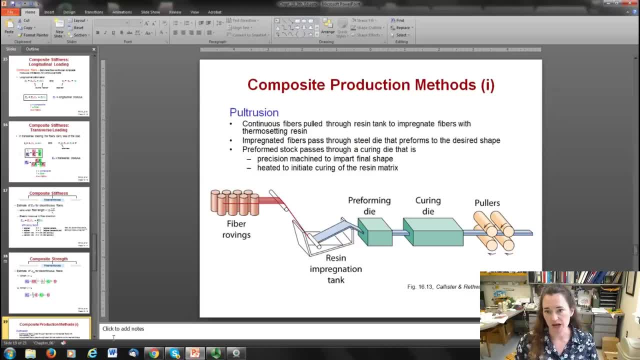 a thermosetting resin, and then those impregnated fibers pass through a steel die that preforms it to the desired shape, and then the preformed stock passes through a curing die that's precision machined to impart the final shape and also heated to initiate the curing of the resin. 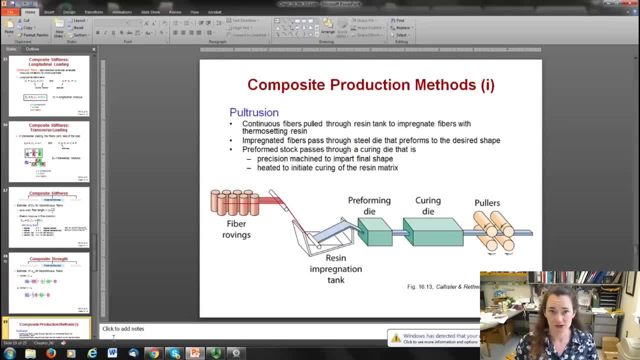 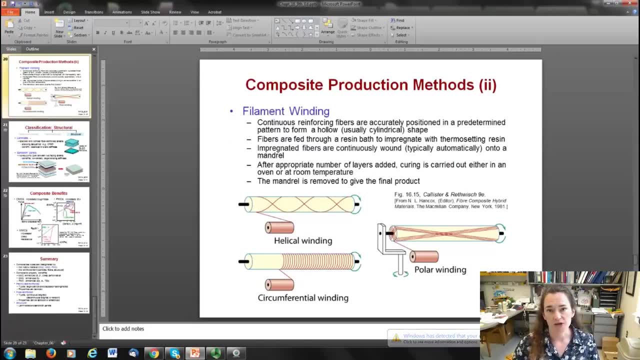 matrix. Now it's actually pretty cool looking when you watch the video, so don't let my rather dull recitation of the facts turn you off from watching it. Another common composite production method is called filament winding, and that's when continuous reinforcing fibers are accurately positioned in the predetermined pattern to 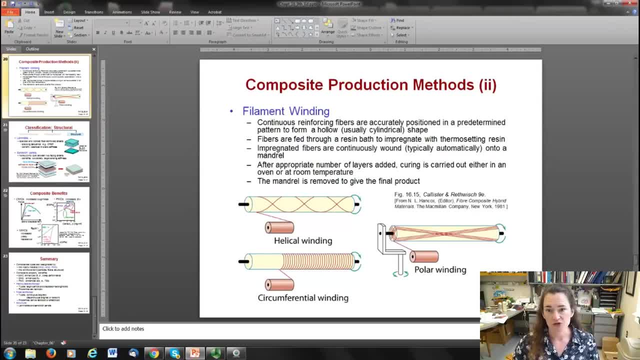 form a hollow, usually a cylindrical shape, And the fibers are fed through a resin bath to impregnate them with the thermosetting resin, and then the impregnated fibers are continuously wound, usually automatically, into a mandrel, And then, after a number of layers are added, curing is carried out either in an oven or 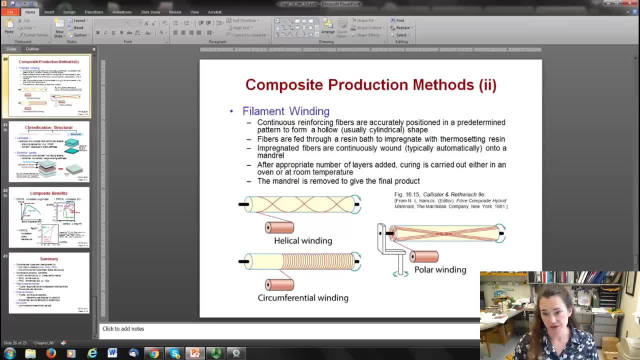 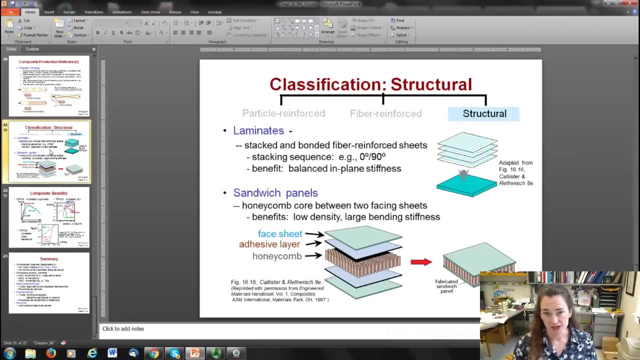 at room temperature and then they remove the mandrel to give the final product, And the animation of that in the video that I posted is really neat to watch. Finally, you're probably pretty familiar with structural composites. You've probably seen them around your house. 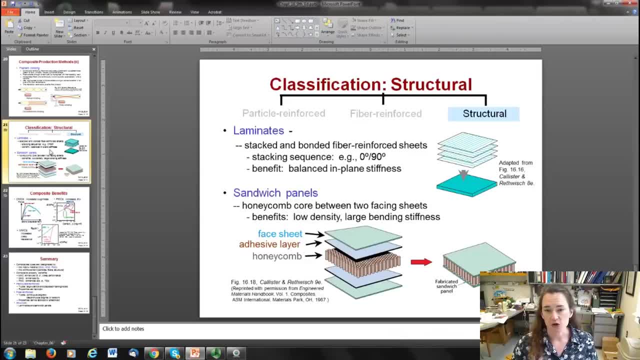 They usually come in two broad types and those are laminates which are stacked and bonded. They come in four sheets. Sometimes they have a stacking sequence. That gets discussed in the carbon fiber for aircraft use video that I discussed, why they choose the stacking sequence that they do. 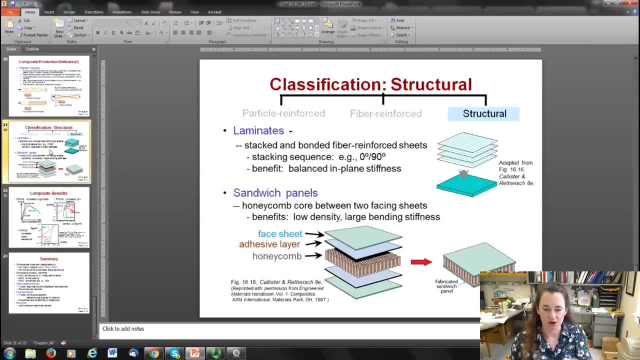 But a really common stacking sequence is to orient. so the fibers are oriented this way in one layer and then perpendicular to that in the next layer, and that provides them with increased tensile strength in either direction. They also have a more balanced in-plane stiffness and they don't have that tendency to kind. 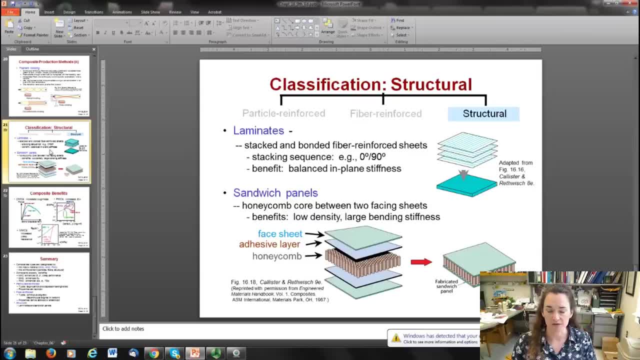 of curl up when they heat or cool that you might otherwise have. You've probably seen sandwich panels and ceiling tiles. That's a really common place to see them And that's when you have a honeycomb core between two facing sheets And the benefits are that they have a low density and they have a very large bending. 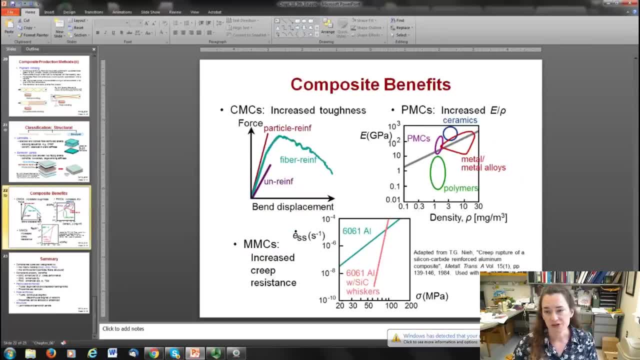 stiffness. So, to summarize, there's a lot of benefits to composites. You can increase your toughness, You can increase your elastic modulus while decreasing your density. You can increase your elastic modulus while decreasing your density. And you can increase your elastic modulus while decreasing your density. 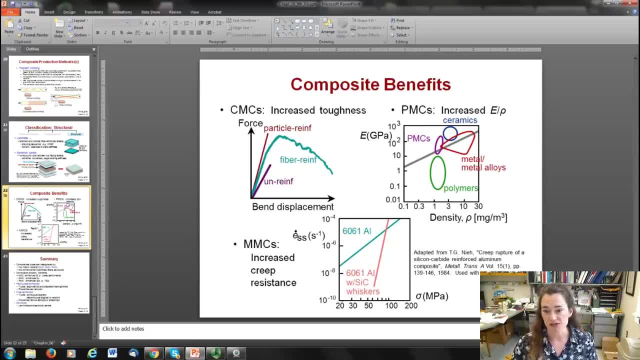 You can increase your elastic modulus while decreasing your density, And you can increase your resistance to creep, which strengthens their performance over time. So I hope you enjoyed that, and be sure to watch all those extra videos that I've posted below for more information. Thanks a lot. 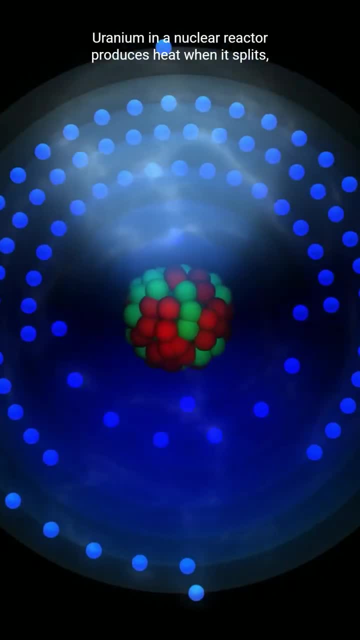 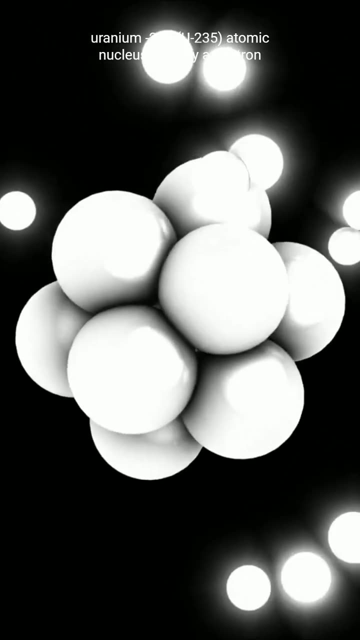 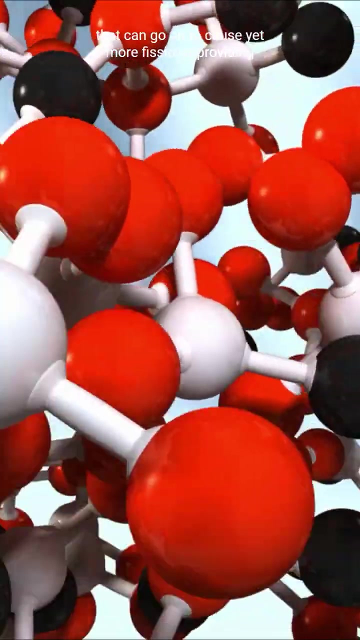 Uranium in a nuclear reactor produces heat when it splits, or fissions, which is what happens when a fragile uranium-235U-235 atomic nucleus is hit by a neutron. At the same time, fission produces several neutrons that can go on to cause yet more fissions, providing a smooth, stable supply of heat.